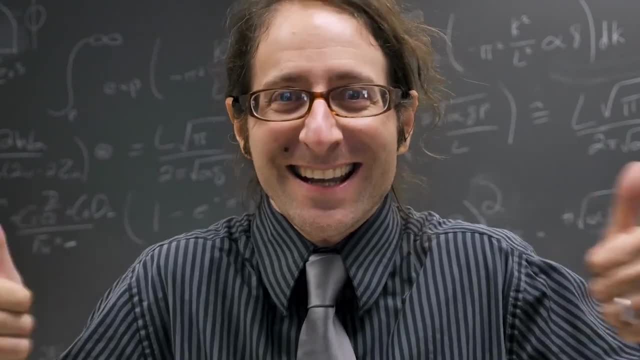 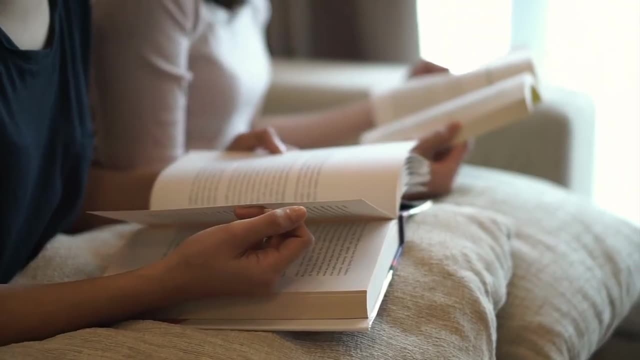 We need to seek them, fill them in and acknowledge that the more we know, the more there is to know. Why will there always be unknowns? This happens because each new book we read will refer to other books, just as each new conversation will reveal details. we've never. 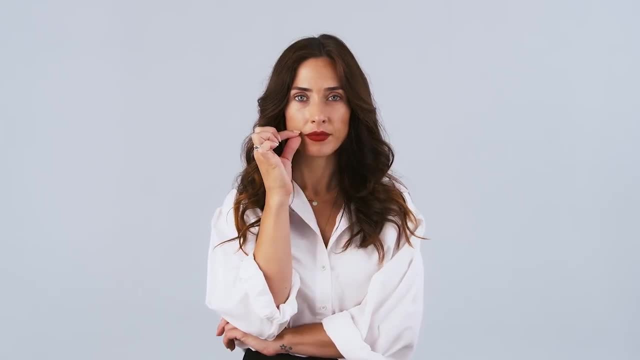 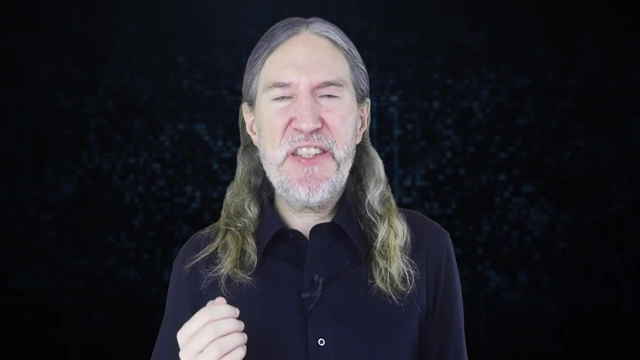 encountered before. Critical thinking also helps us avoid traps such as being a know-it-all, when the only thing we know is that we can't know it all. And if we do make that mistake, critical thinking gives us the modesty needed to admit when we're wrong Now, instead of being 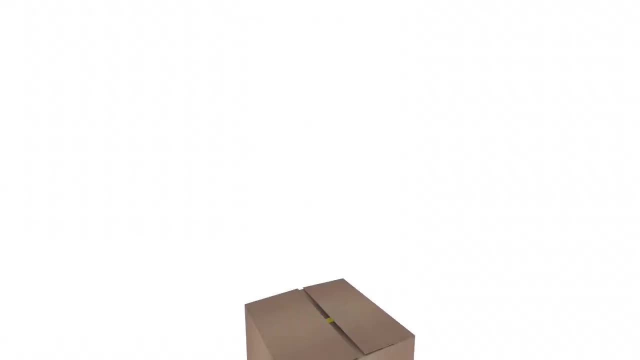 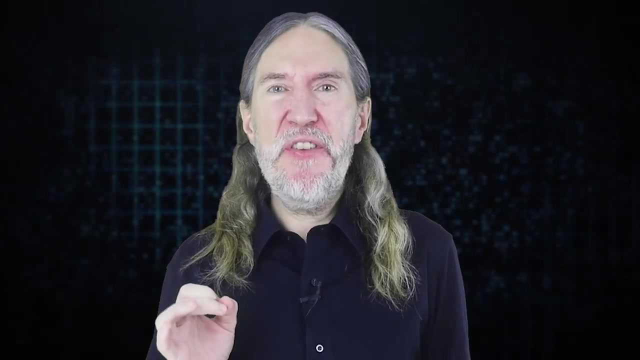 humble. lots of people skip around and dance and then make some vague claim that you have to be willing to think outside of the box. This is sometimes true. More often, however, people haven't thought their way through the inside of the box nearly enough. But, as you'll see from our 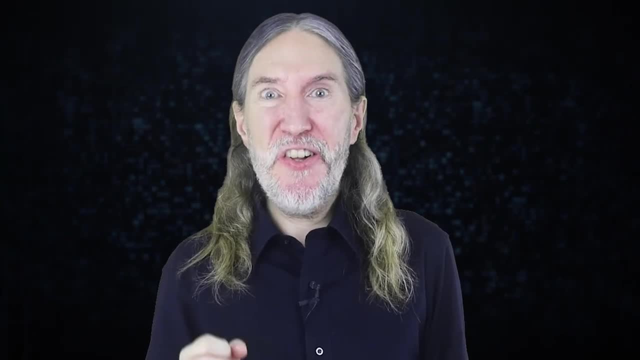 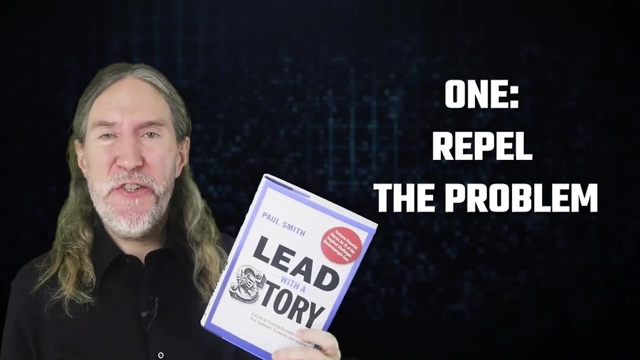 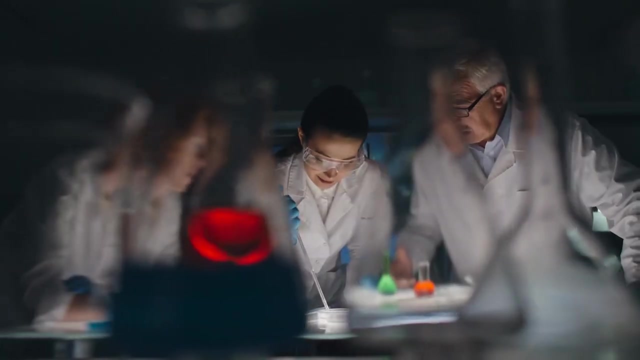 first example. sometimes you have to get rid of the box altogether. In Lead with a Story, Paul Smith relates the tale of Tide, a laundry detergent brand First introduced in 1946, the brand's owner, Procter & Gamble, sought to improve the product. They spent years trying. 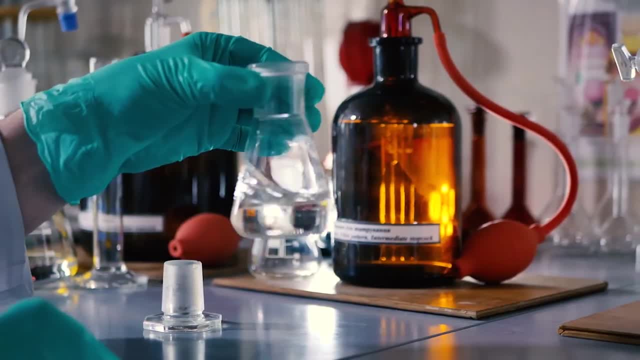 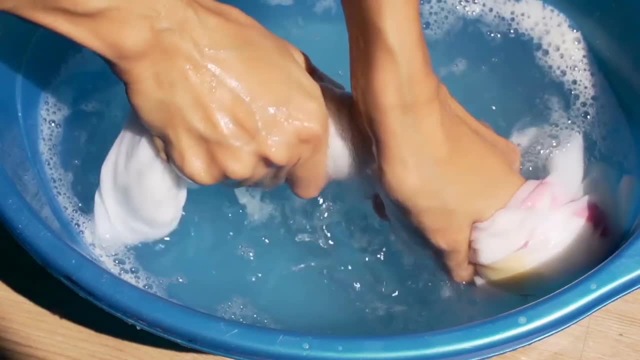 to create formulas that would remove tough dirt stains without damaging clothing. It turns out there is no way to make a detergent stronger without also weakening the fabric it is made to clean, unless you have great minds on the team to work through such critical thinking scenarios. 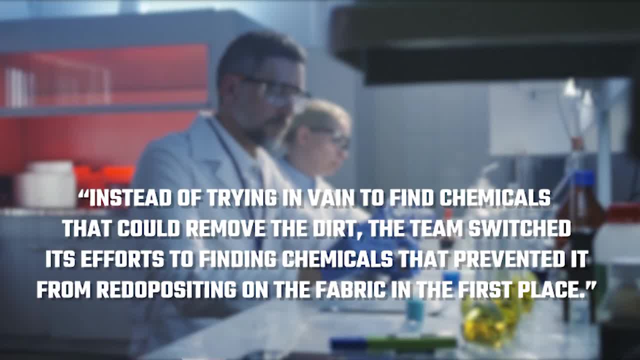 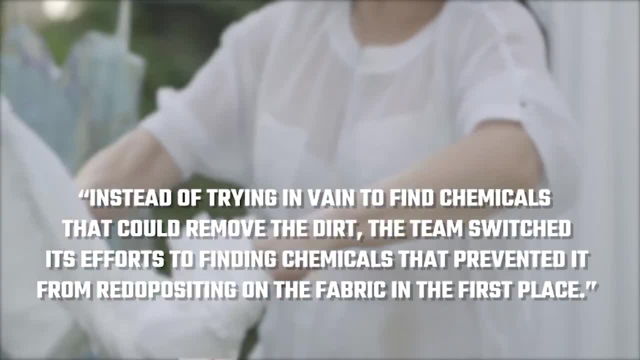 So, as Smith sums it up, instead of trying in vain to find chemicals that could remove the dirt, the team switched its efforts to finding chemicals that prevented it from re-depositing on the fabric in the first place. In other words, the Tide team found a way. 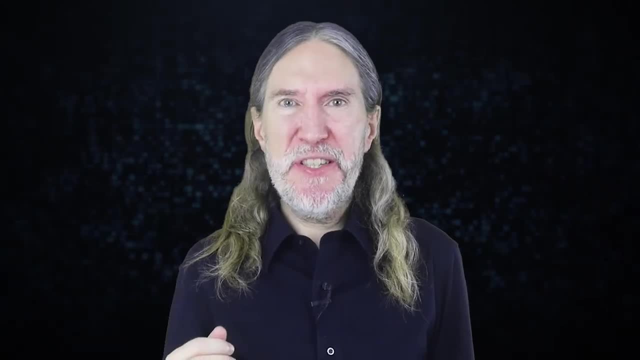 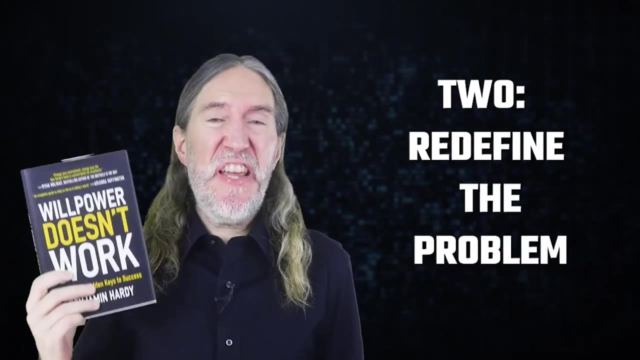 to prevent the problem of clothes getting dirty in the first place, And that's what I mean by sometimes- you have to throw the box away altogether. Benjamin Hardy named his best-selling book by saying the problem out loud. willpower doesn't work, And we all know this from experience. 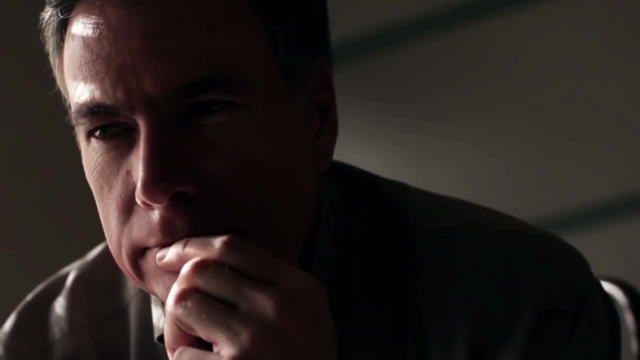 We try to use our minds to motivate ourselves, but continually fail. But by looking at a few factors such as the neurochemistry of the brain and what seems to be the most important part of the brain, we can see that the brain's most important part of the brain is the brain, Instead of what successful people actually do. 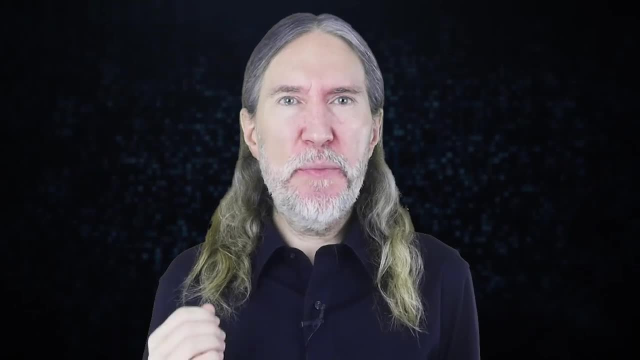 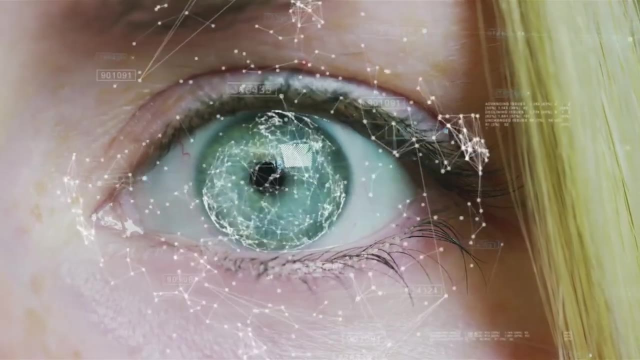 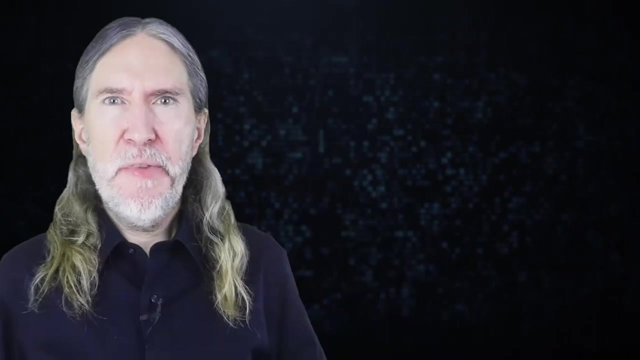 instead of what we imagine they do. Hardy identified the rules and principles that govern the environments of successful people. So, instead of battling a problem that can't be solved, like willpower, use science to redefine the problem and build environments and performance systems that make success inevitable. In The Luck Factor by Richard Weissman. 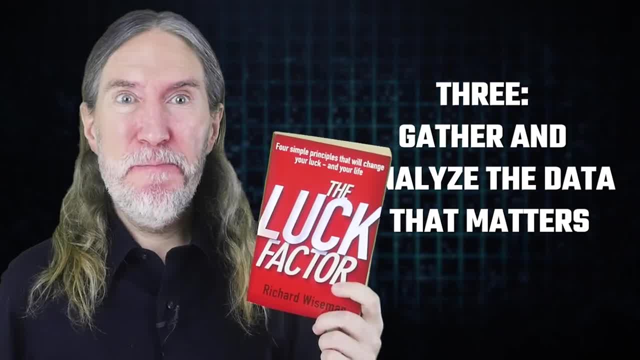 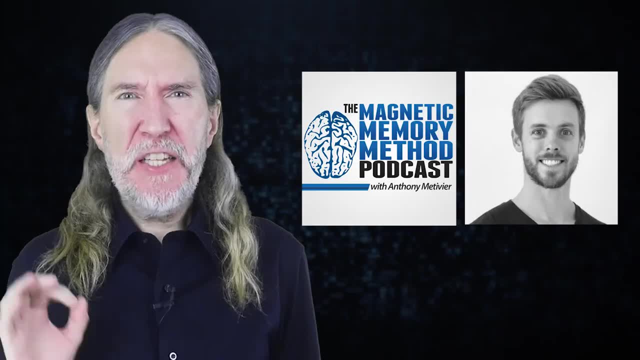 you'll read the story of Carolyn, who felt down on her luck. Rather than leave things to how Carolyn felt, Dr Weissman had her fill out a life satisfaction questionnaire. It's much like the Wheel of Life I discussed with Arthur Worsley. 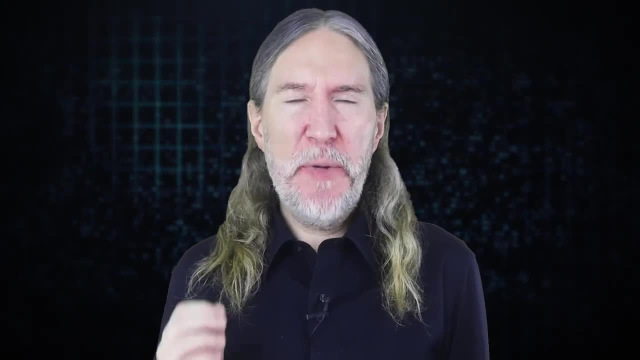 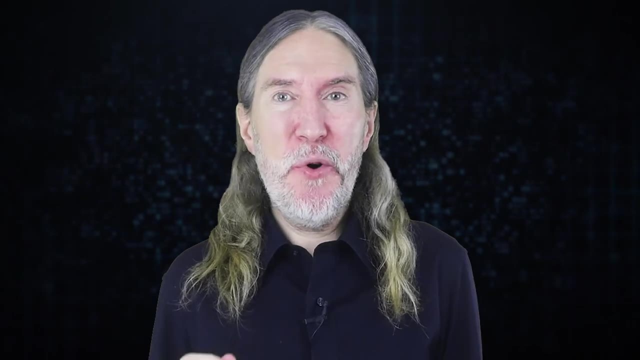 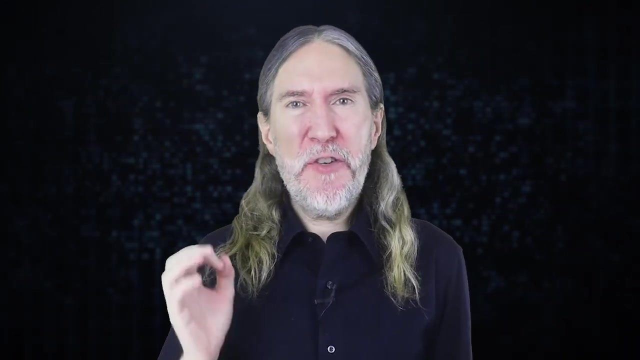 on the Magnetic Memory Method podcast. After getting the data down on paper, Dr Weissman gave Carolyn some lessons in how to be more lucky in life. Spoiler alert: most of those lessons involve little more than reflective thinking and objective reasoning, two key parts of thinking. logically, you might want to beef up on After applying these principles. 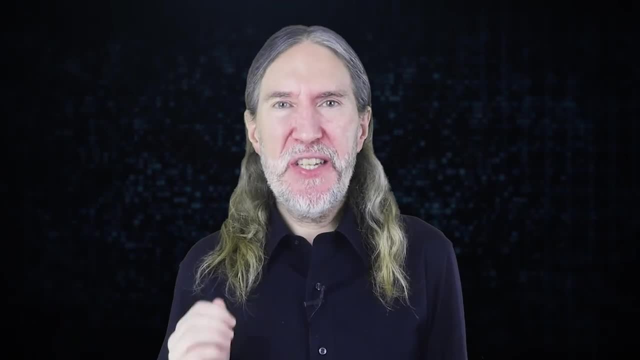 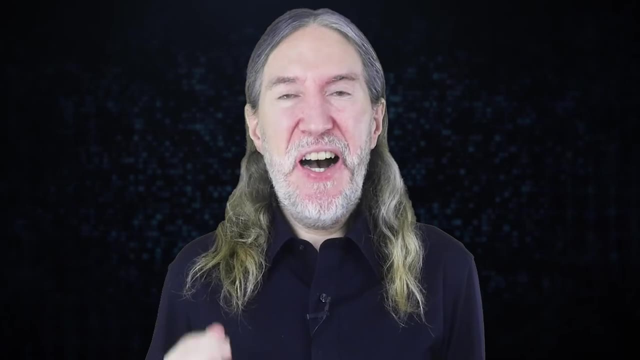 Carolyn's luck went up, as did many other participants in Dr Weissman's studies. This book changed my life. Prior to completing its exercises and analyzing my own data, I had a very bleak outlook on just about everything in life. But when you think critically about the data that matters, 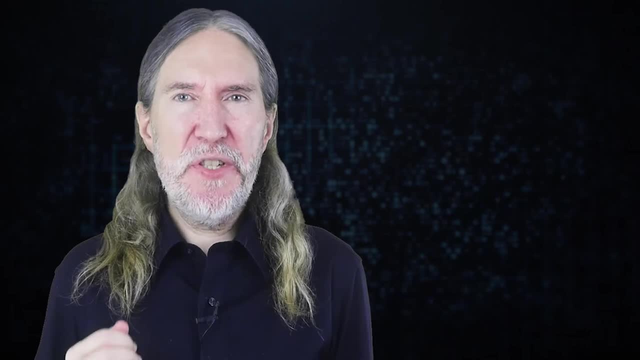 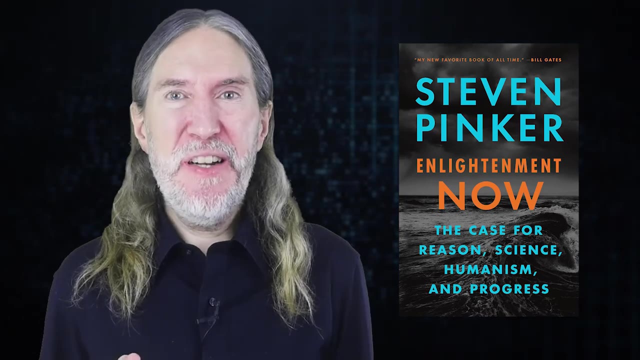 it's much easier to see ways to improve your life. So for more science-based examples, see the data behind why the world itself is getting luckier in Enlightenment Now by Steven Pinker and Factfulness by Hans Rosling. And when you analyze data, you're going to discover some. 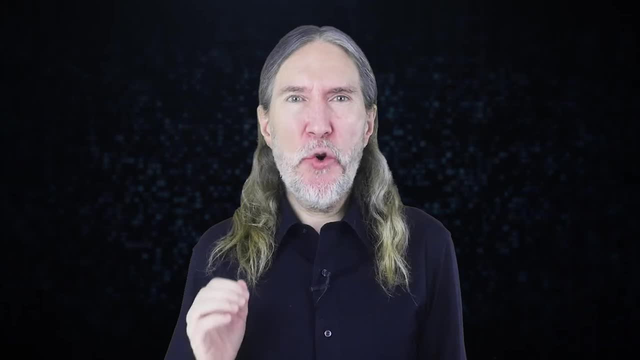 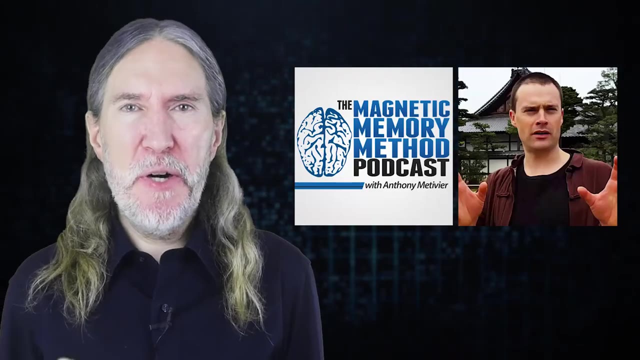 uncomfortable truths, But as an advanced thinker, it's your duty to point your findings out in a calm and kind manner. This was the case when I interviewed fellow mnemonist and memory expert Martin Fox. In our discussion he used Sherlock Holmes as 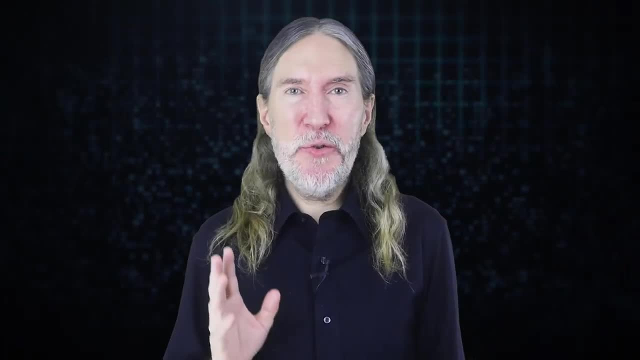 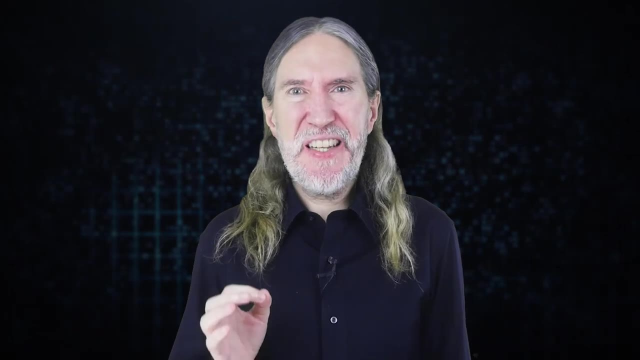 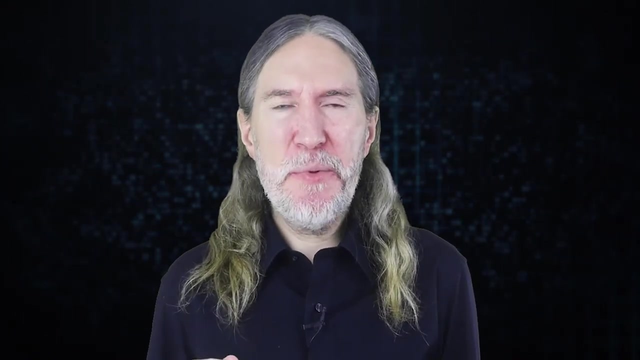 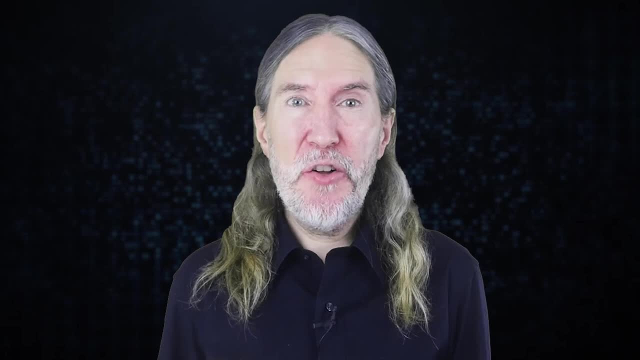 narrative world is associated with the idea of memory palace And this narrative world is associated with the idea of memory palace And this narrative world is associated with dark themes of criminal murder and not at all related to the positive outcomes. we actually use the techniques to 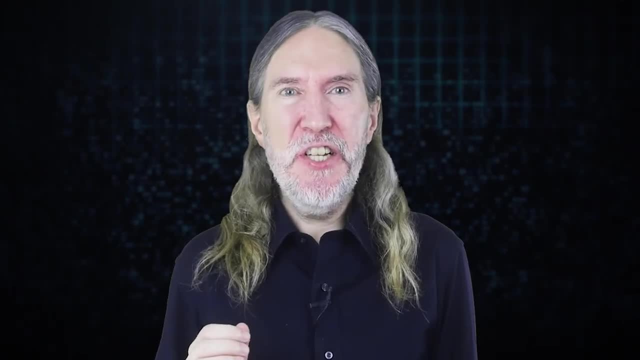 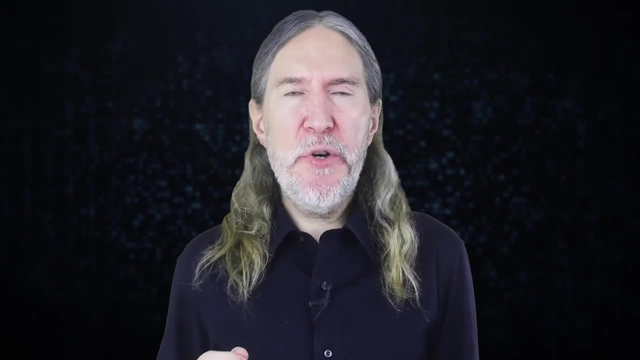 achieve, And Martin wasn't offended at all. In fact, it opened up the discussion to a new and unanticipated area both our audiences enjoyed. So, in sum, always speak plainly, without trying to avoid or erase issues you fear might be unpleasant. To do so is the opposite of critical thinking. 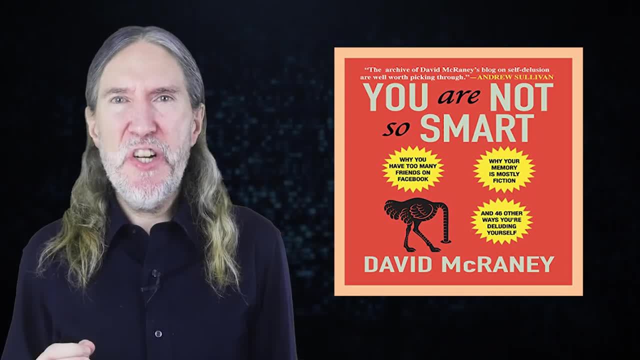 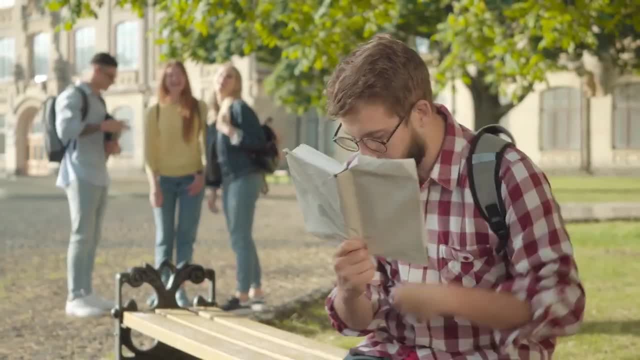 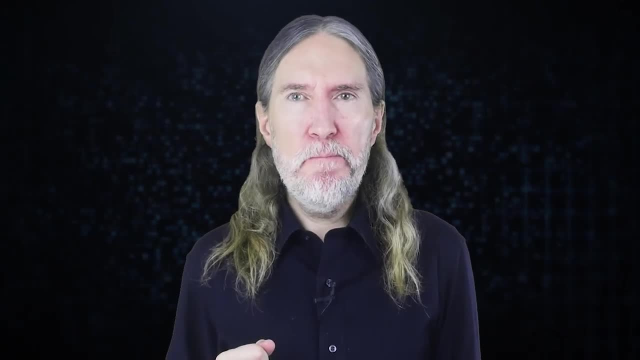 Yet how many of us berate ourselves by worrying about what others think about us? For example, some of us engage in self-punishment for hours when we've said something we think is stupid. We unfortunately don't realize that people simply forget the vast majority of what we tell. 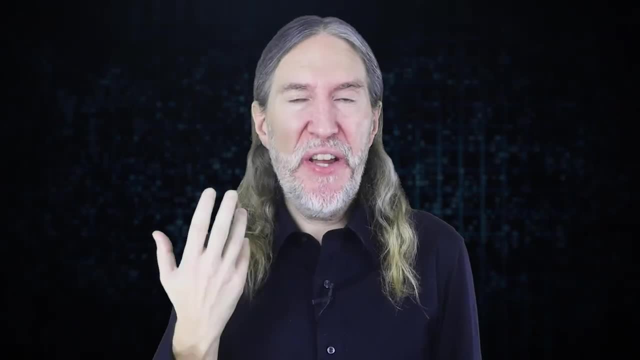 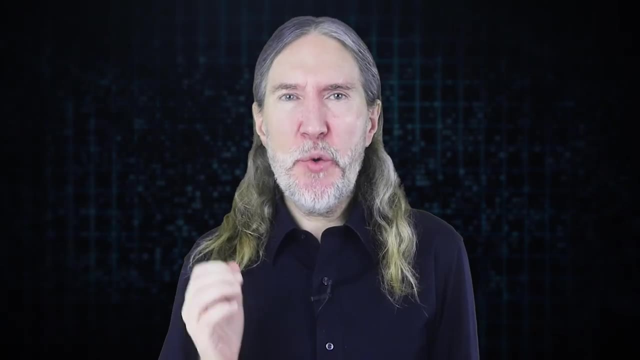 them. Likewise, if you have some dead skin on your face, like I deal with every single day, or dirt on your clothes because you don't use Tide, most people either won't notice or forget about it quickly. Darren Brown makes a similar point in his book Confessions of a Conjurer. 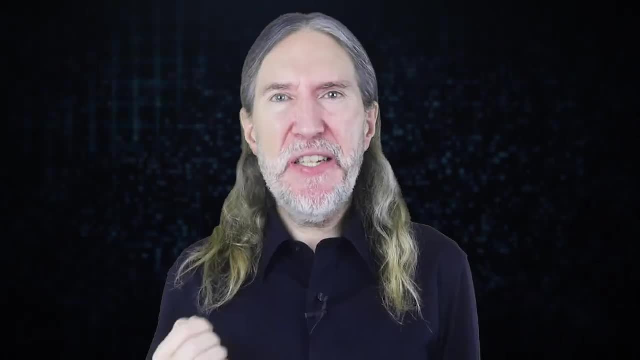 In this book, Darren Brown talks about self-punishment and self-punishment. In his book, Brown talks about a friend with poor skin. His friend did not realize this psychological fact about how quickly people forget about their attention span and their bad memory. 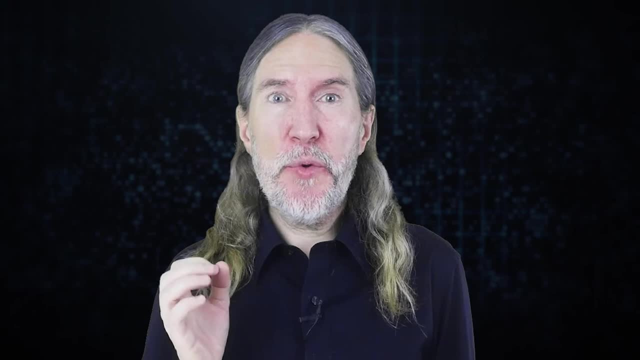 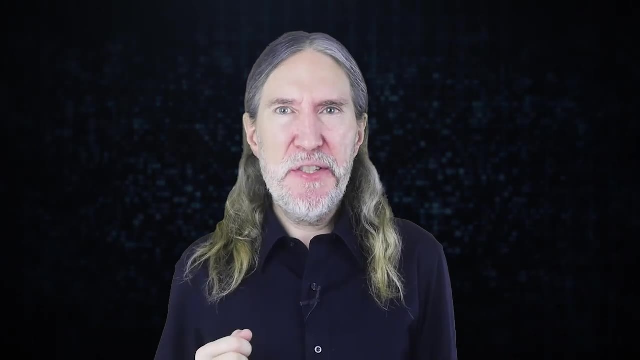 As a result, this person tortured himself unnecessarily with worry about what other people think. Not only can you remove yourself from such suffering, but you can improve your own thoughts about others, As Brown goes to great pains to point out in his book. if we are the kind of people who would judge others over such fickle matters. 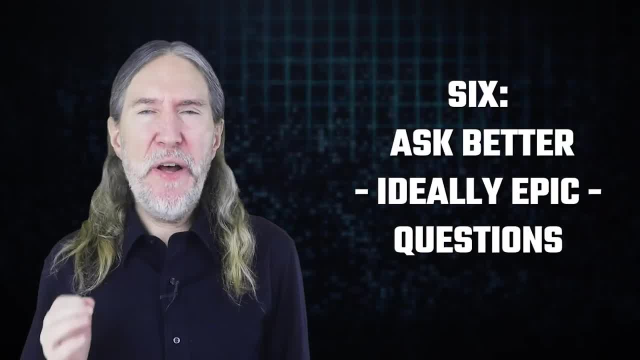 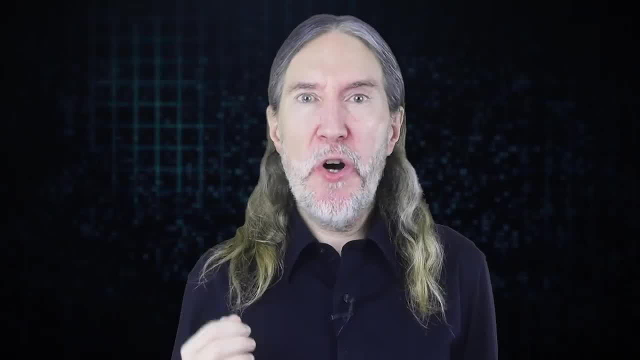 we should learn to be more kind. In his famous essay What is an Author, Michel Foucault asks us to go beyond right and wrong. For example, both Sigmund Freud and Karl Marx were wrong about many things, and in both cases, 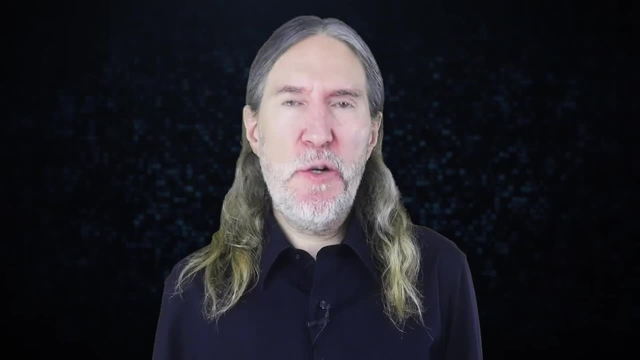 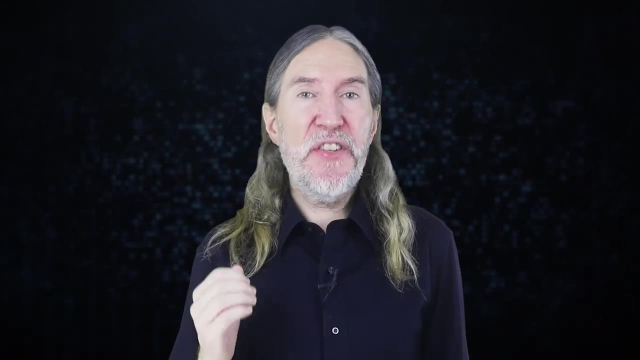 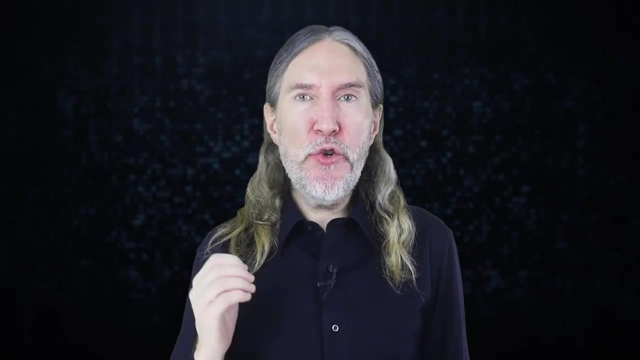 many tragic outcomes resulted from the mistakes in their works, But by the same token, they opened up new conversations that people were not able to have before. Obviously, there's a lot at stake when asking questions that change the nature of entire societies. Elon Musk is one such person, asking new questions in our era and influencing change. 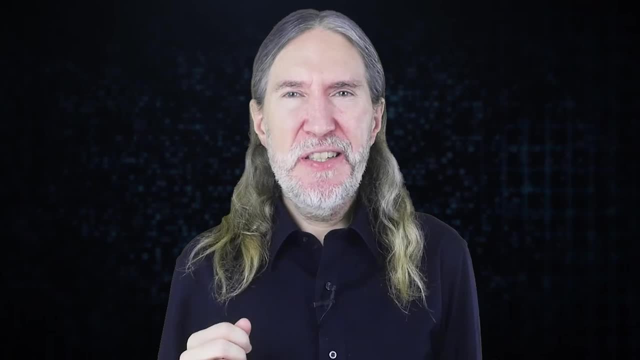 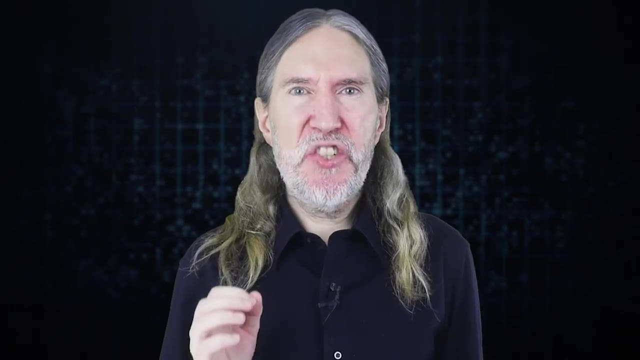 as a result, Despite his talk of first principles thinking, he's not always the greatest demonstrator of this kind of model. But, as Foucault points out, we need people like this to take the risks and take us into new areas of thought. Then we can study their examples and 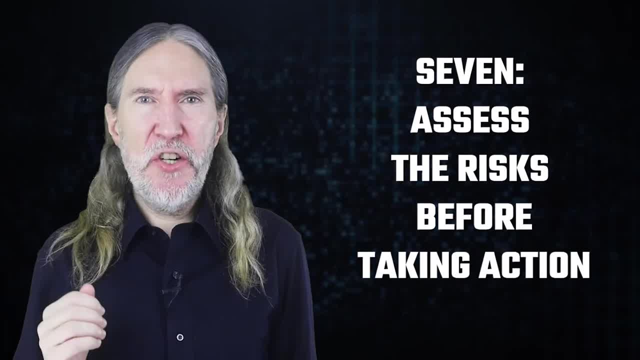 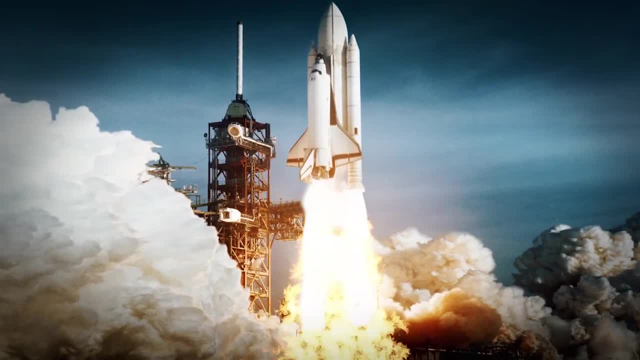 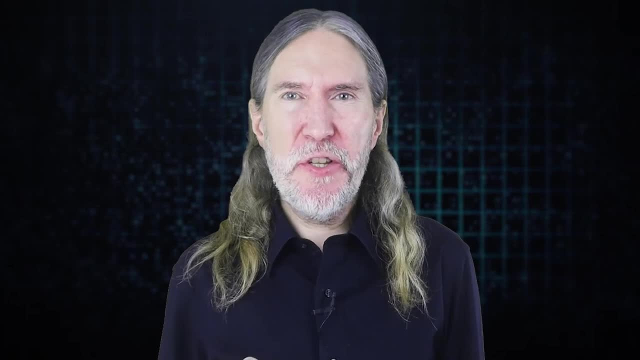 do better in the future. Perhaps no organization on Earth is better at assessing the risks than NASA. They've sent people to the moon and helped maintain an incredible international space station. You can actually read their risk management handbook. Not everything in it will apply to your life, but you can still learn a lot. For example, 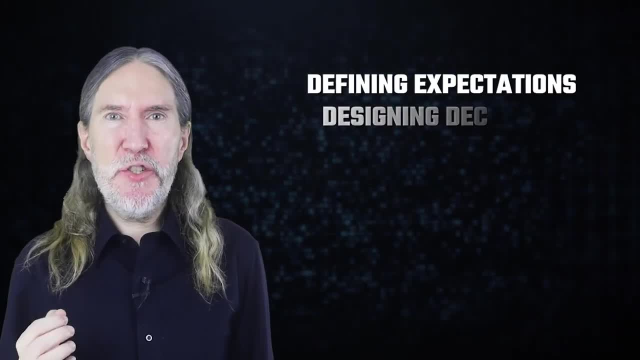 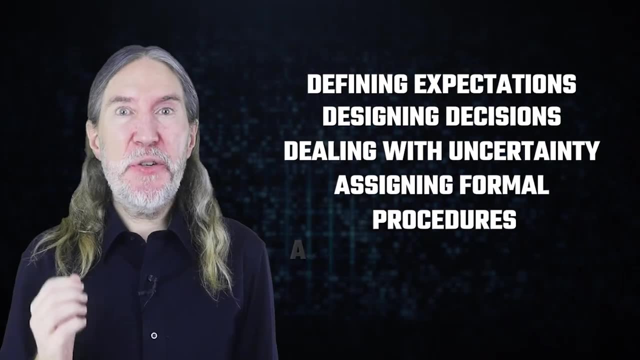 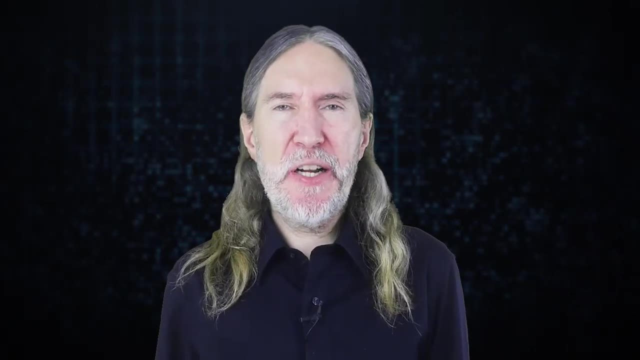 you'll learn about defining expectations, designing when decisions will need to be made and how to make them, dealing with uncertainty, what kinds of situations require more formal procedures and how decision makers should act and to whom they should be responsible. But if this kind of material direct from the source is too abstract, 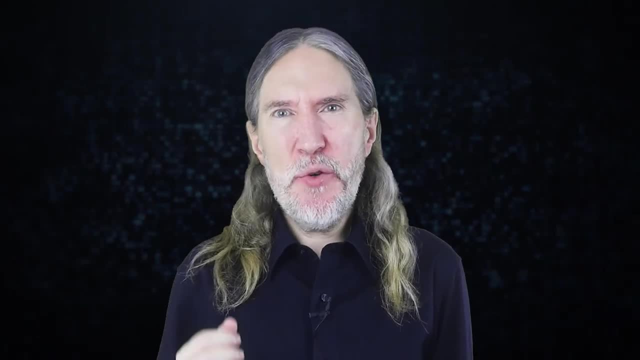 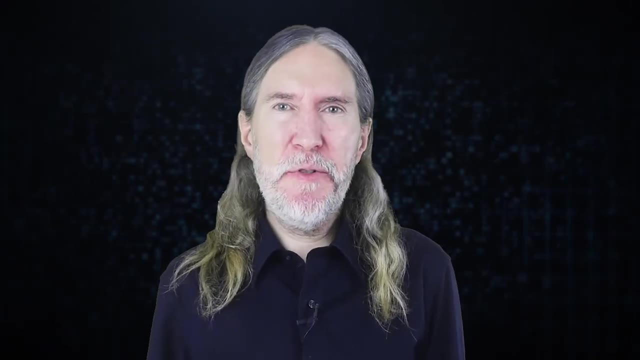 there are many wonderful books about various NASA missions that give you a strong sense of the critical thinking involved. The First Man by James R Hansen is an incredible read, to take just one example. So how do you get started with thinking more critically? Well, let's get into it, But first. 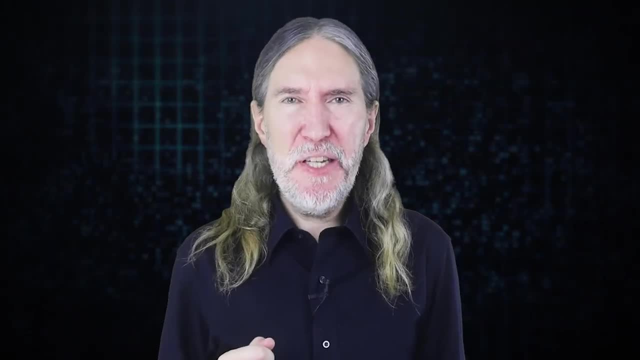 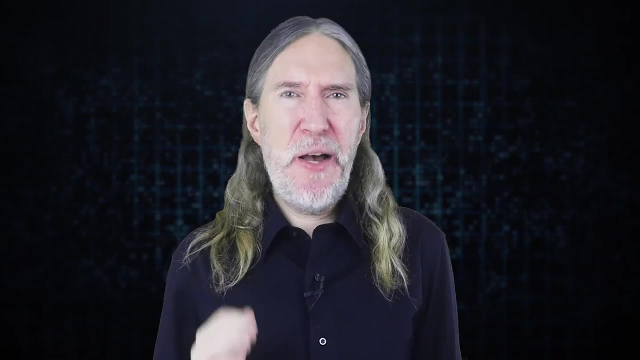 I want to thank our channel members and everyone in the Magnetic Brain Method family. You make all of this possible, And I especially love when one of you asks for material like we're covering in today's video. So if you want more, let me know loud and clear. Hit that thumbs up. 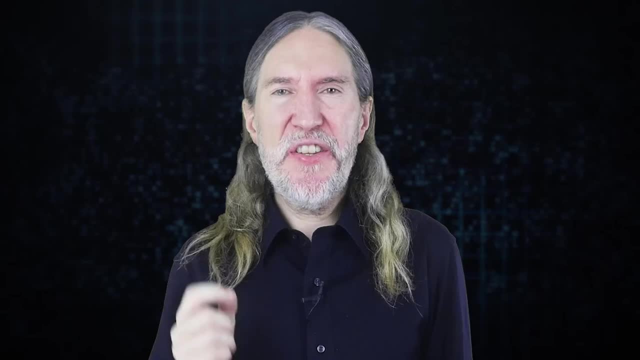 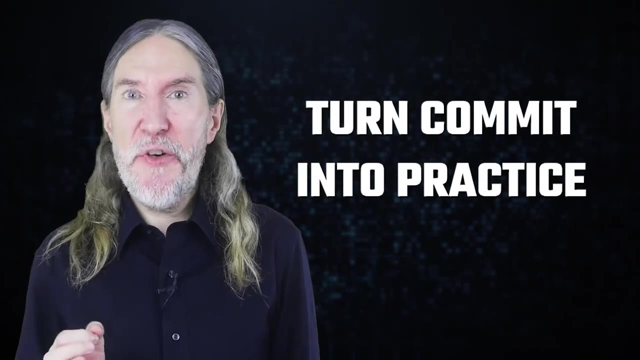 And if you're new here, get subscribed. Now, when it comes to starting to think more critically, I'd suggest that the first step is to commit. Commit to what? To practicing the art of thought and to the art of thinking, And that's pretty easy. You can start writing more often, That's. 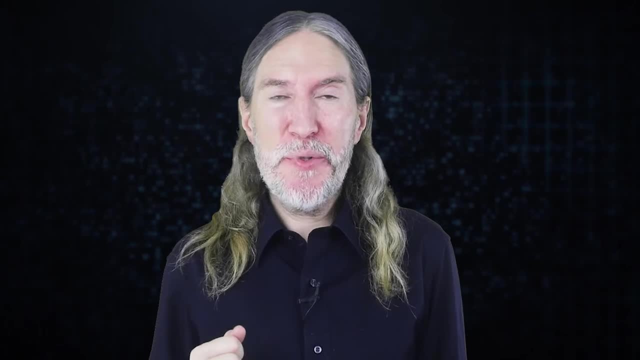 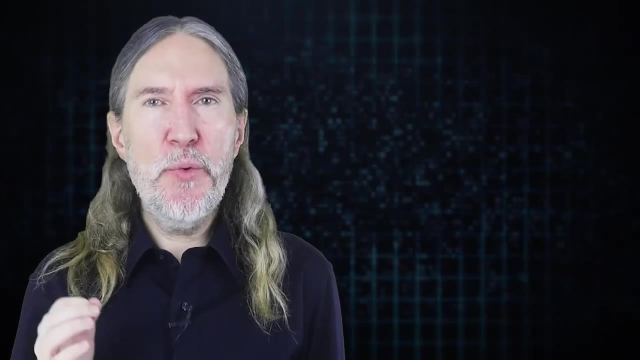 pretty easily done when you read more often. I've given plenty of examples you can read in this video and I hope you'll follow up with some of those books. Next, you'll want to start writing as much as possible. This will create metacognition. 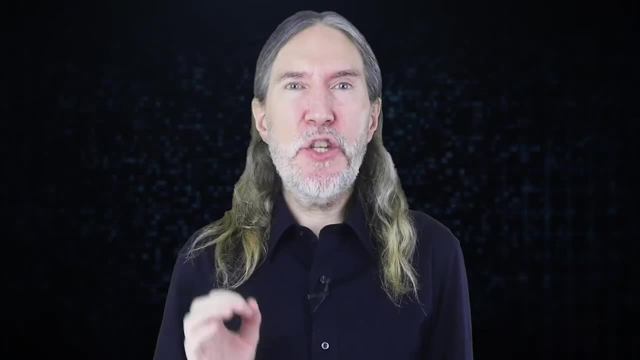 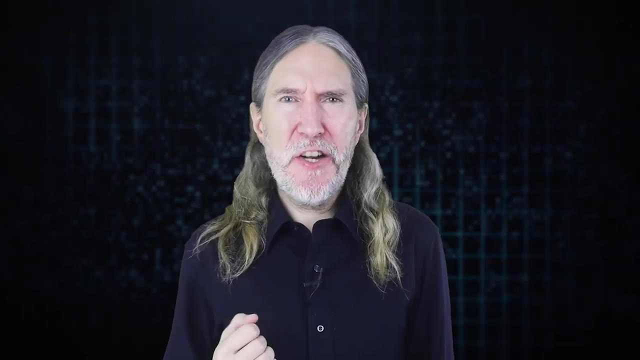 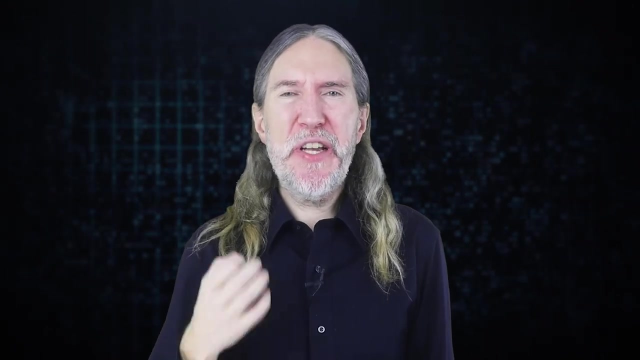 because writing is known to create thinking about thinking, especially as you engage in the meanings of words and the use of examples at a higher level. Finally, discuss much more often and discuss at length. Instead of one sentence, comments on videos. instead of one answer, responses. push yourself to explain at greater length. 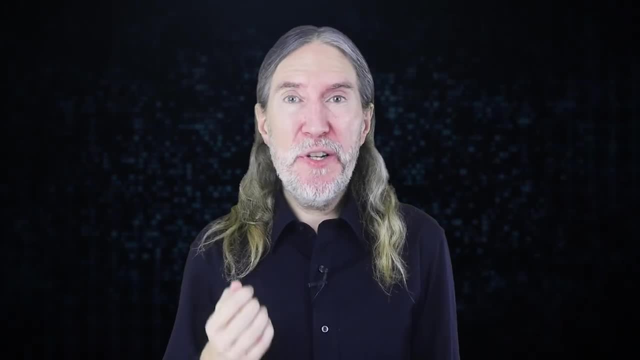 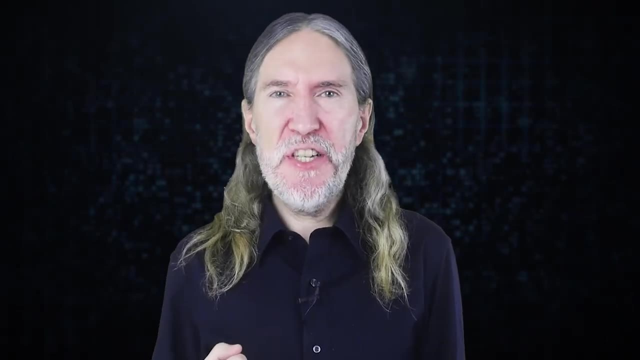 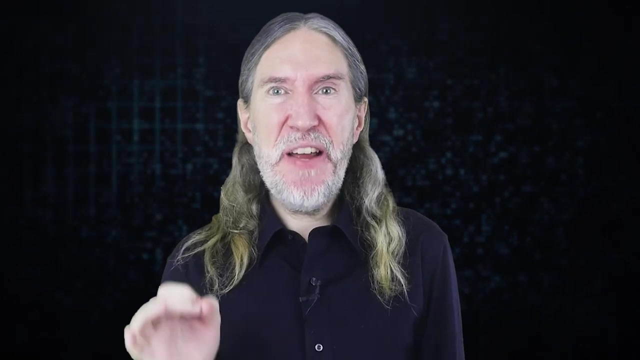 and bolster what you say with examples that support what you're expressing. Never rest on your opinion, Always supplement with research findings from your reading, from other conversations you've had, and question everything as you continue to question yourself and the status of each and every question itself. That's what critical thinking is all about.